Okay, so critical render path: advanced CSS in the advanced CSS section and that is part 53.. So once I reach out my memory and what happens in that, But I will let you know and we can move on to the next one. Okay, See, ya. Okay, so critical render path: advanced CSS in the advanced CSS section and that is part 53.. So once I reach out my memory and what happens in that, But I will let you know and we can move on to the next one. Okay, See, ya. 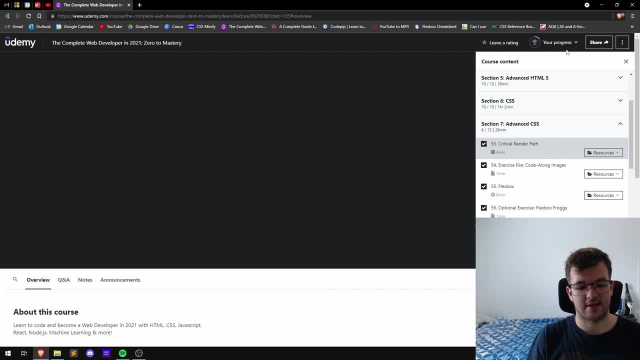 It's basically the path that the website takes to load. So when you write the web address in the top bar, it goes out and looks for the server and the server gives it the HTML file first of all. Then it starts reading. if there's CSS in it, It will also tell the server: please give me CSS file, And it will get them. if there's, let's say, a text font styles that you would like and you have defined where it's from. 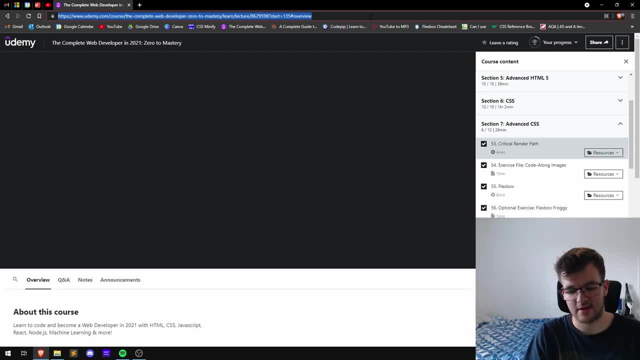 It will then grab that inside the CSS as well And basically the critical render path is just the way you go about doing this and ways of possibly decreasing the path and speeding up the process of loading the website. So one of the ways is by using 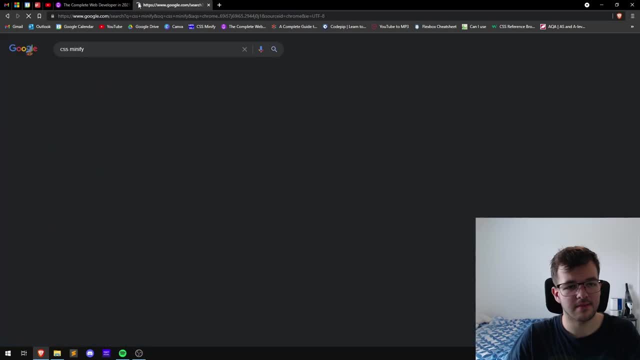 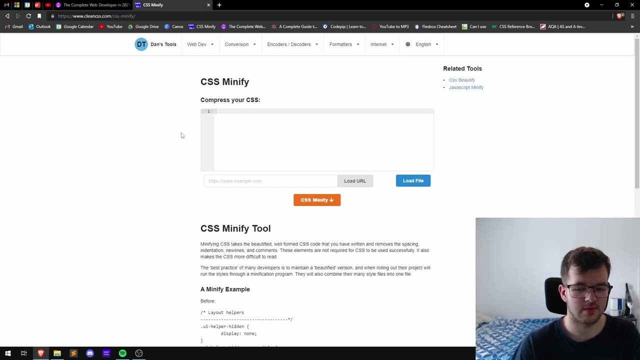 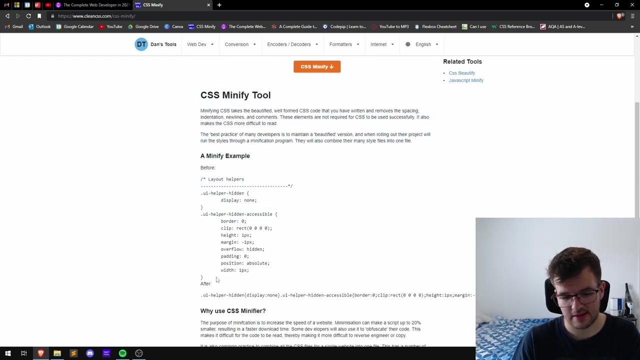 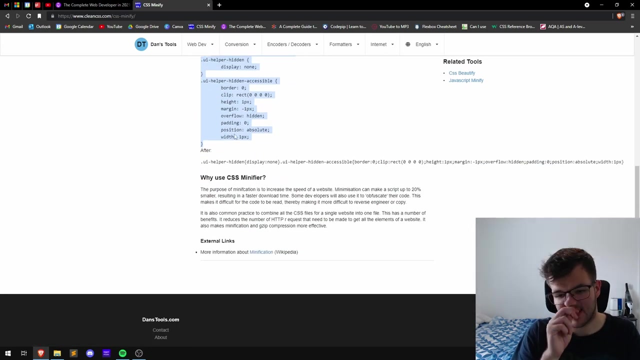 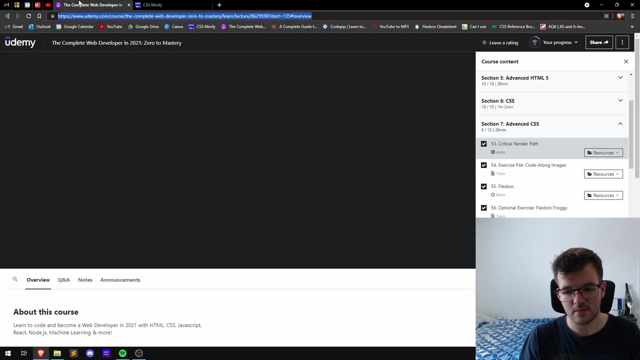 CSS Manify, which is a tool that people who program use to create examples like this of CSS into examples like this: taking out all the white spaces and making it more compact, using less data that needs to be sent over the internet. There's not much else to it. 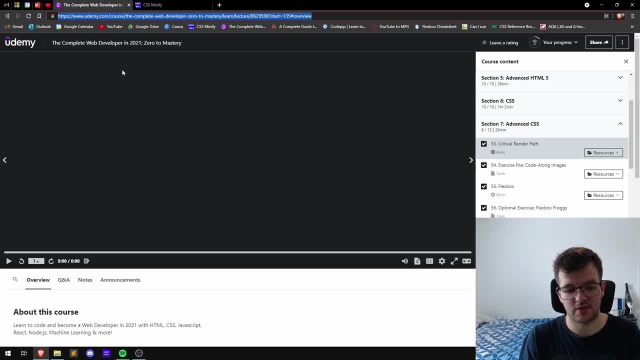 It's also good to consider The size of the CSS HTML and where you're getting the font that you're using from, just so, And if any images you're also taking from the web, you need to make sure how reliable and fast you can get them to your website so that they load as soon as possible.